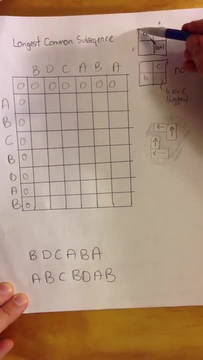 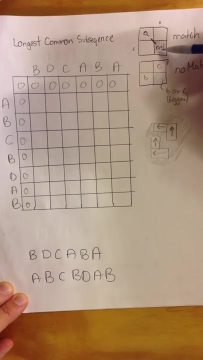 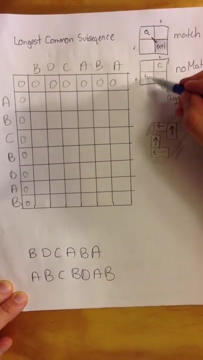 If this value and this value is the same, There is a match, Then we are taking a number from this cell, Adding one, and we are inserting the answer here. If there is no match, Meaning when this value and that value are different, then we are considering those two values. 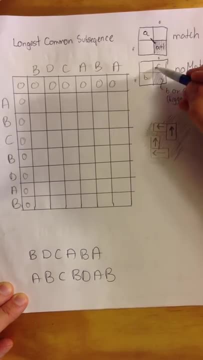 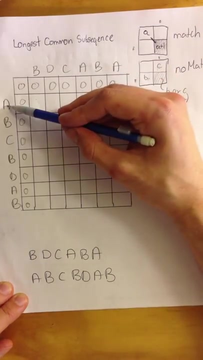 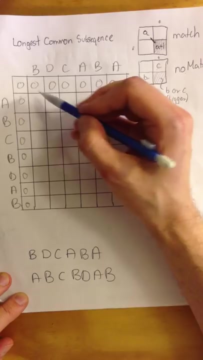 and inserting here the biggest one out of those two. So let's see how it works. We are here, We are comparing B and A. They are different, so there is no match. There is no match. We consider those two numbers. Which one is bigger? 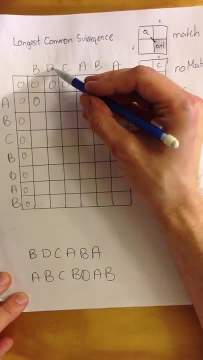 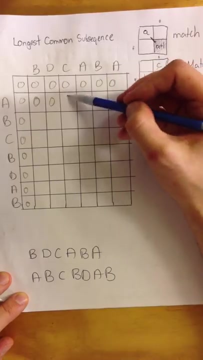 Both are zeros, So we are putting zero B and A Again. the same situation. We compare those two Zeros, So we put zero C and A Again. Now something interesting happens, So we have A and A. There is a match. 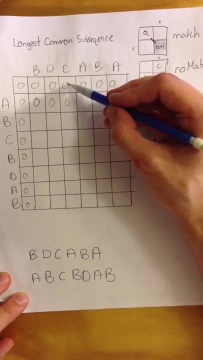 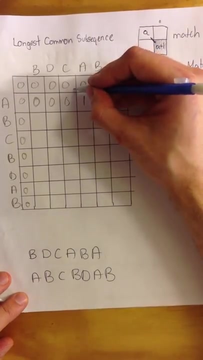 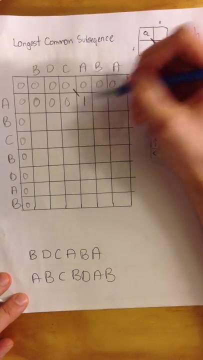 What we do is we look at this value And we are adding one and inserting a number over here On top of this. we are creating here a bridge, So we just create a connection between those two values which are indicating that there was a match. 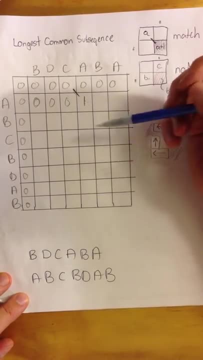 Later on I will tell you how to do it, How we are going to use this bridge later. Ok, Let's keep going. So we have B and A. There is no match, And so we compare those two values. This one is bigger. 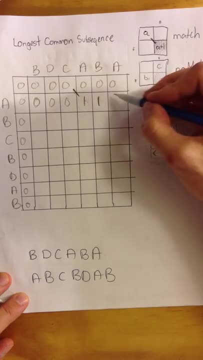 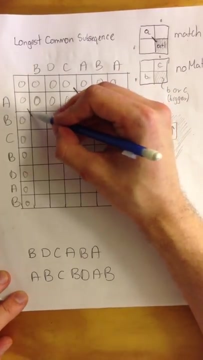 So we are putting one A and A Again match. We are creating a bridge, We are taking this value Adding one, Putting one B and B Match. Bridge Zero plus one is one DB. No match, Bigger is one. 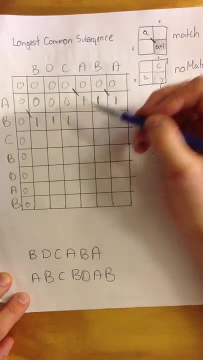 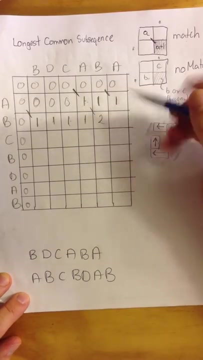 CB- No match Bigger value is one NA NAB- No match Bigger value: one BB Match Bridge One plus one. Two NAB- No match. Biggest value here is two B and C. 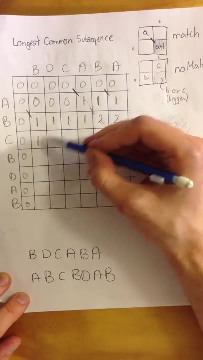 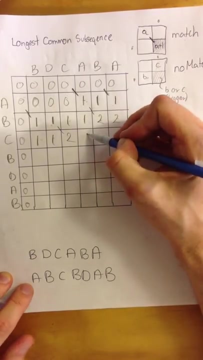 No match: Biggest value: one D and C. No match, Biggest value is one C and C. We have a match, We create a bridge. One plus one is two NAC. No match, Biggest value: two BC. 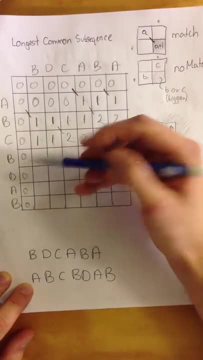 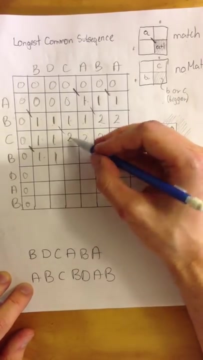 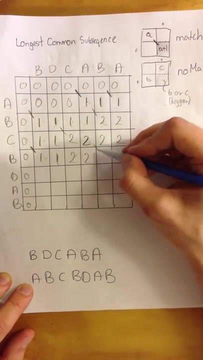 Biggest value: two NAC- No match. Biggest value: two BB Match. Put bridge Zero plus one. One BD- No match. One CB: No match. Two AB No match, Two BB. We have a match. 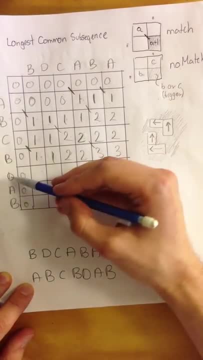 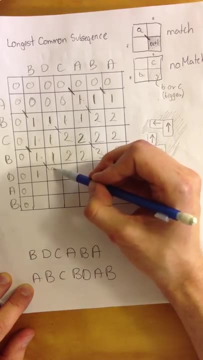 Bridge. Two plus one is three: NAB- No match. Biggest value. three: BD- No match. Biggest value. one: DD- No match. One plus one Plus one is two: CD- No match. AD- No match. 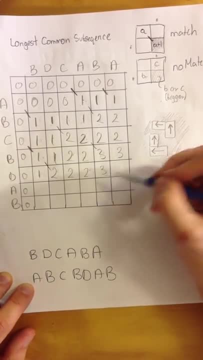 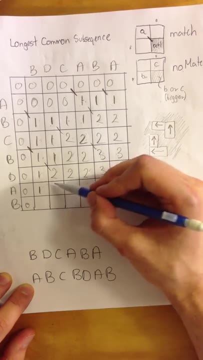 Biggest value: two BD: No match Biggest value three: AD: No match. Biggest value three: BA: No match. DA- No match. Biggest value: two: CA: No match. Biggest value AA. We have a match Bridge. 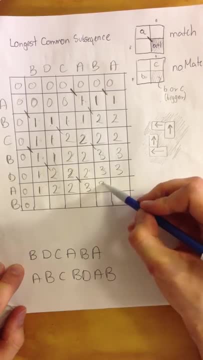 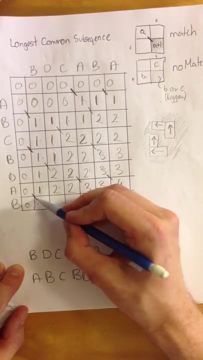 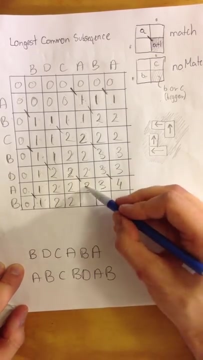 Two plus one Three BA: No match. Three A match. Bridge. Three plus one Four. The last row BB Match. We have a bridge Zero plus one. One BD: No match, Two CB. 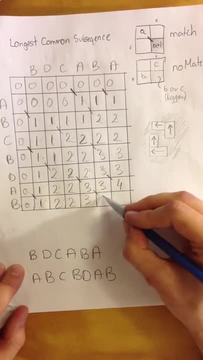 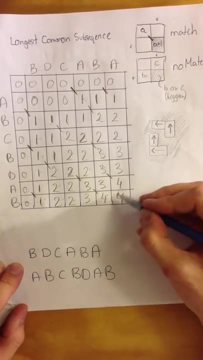 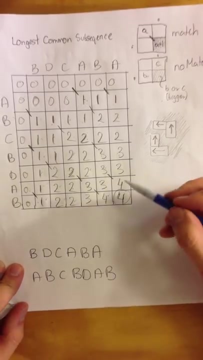 No match. Two AB: No match. Three BB: We have a match. We create a bridge. Three plus one, Four AB- No match, But the biggest value is four. OK, So We have left two letters in the longest common sequence. 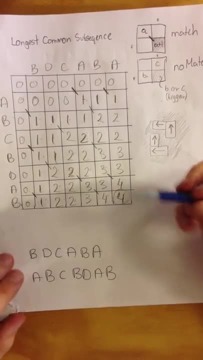 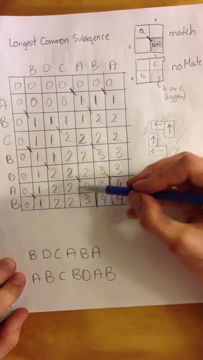 But what are those letters So? So Now we have to backtrack, And so there are two things that we have to see. So First one is that, Actually, By filling out this Table, We created those kind of islands of letters. 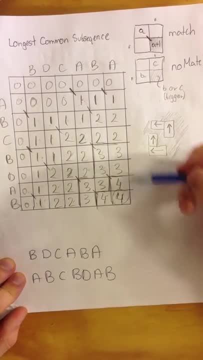 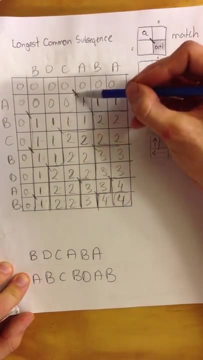 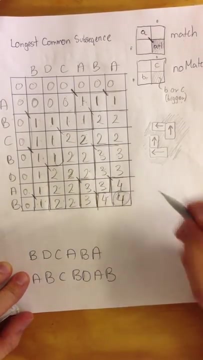 I mean of numbers. So Here are fours, Here are threes, Here we created island of twos And here it is area of of ones, and on the end is a kingdom of zeros. so we are starting over here. what we're gonna do. 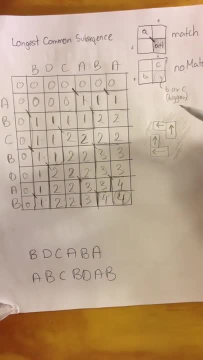 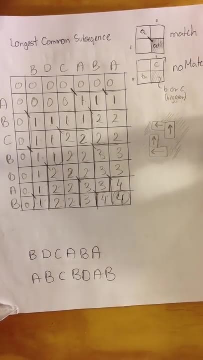 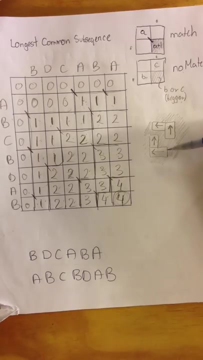 is we have to travel to zero till we are reaching the zero, and we can go to left and top or to the top and left, and we have to be consistent through our journey. so we have to select on the very beginning how we want to go, and so let me select this one: left and top. so the first thing we do